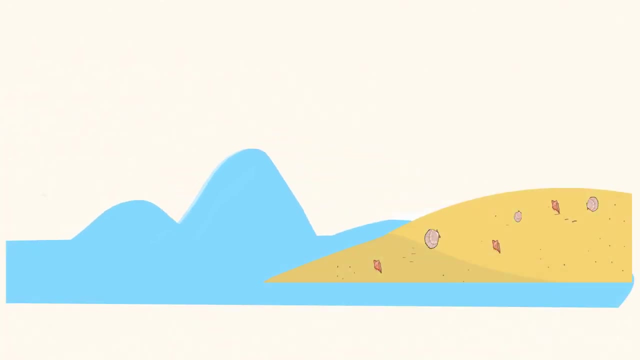 As ocean waves get closer to the shore, the water gets more shallow And this causes the waves to slow down and get closer together. When this happens, the wave length gets smaller and the height of the wave increases. Waves in the ocean Is a lot of fun, but we have much more to investigate on land. 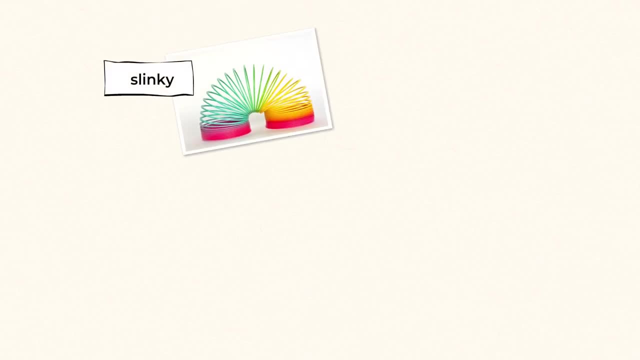 Ohhhh cool. This toy is called a slinky and it's perfect for learning about the way that waves, especially sound waves, work. Watch what happens when one person moves their side of the toy. Ha, ha, ha Wow. 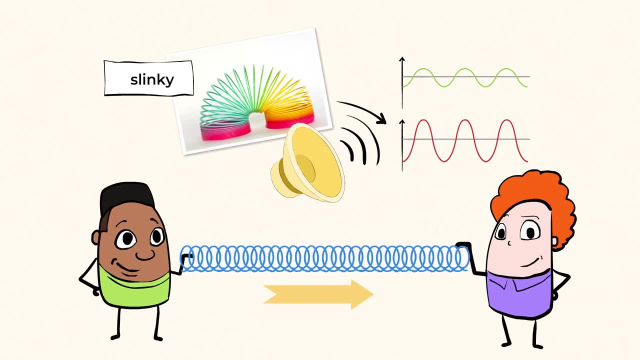 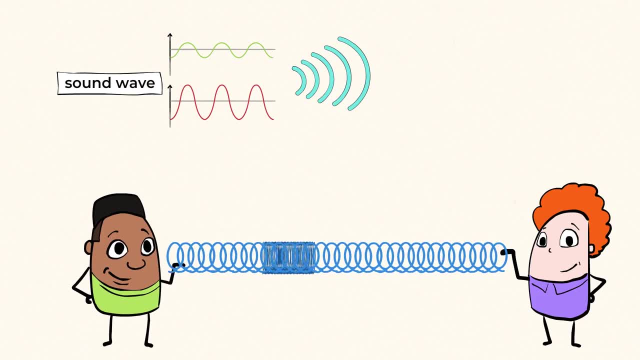 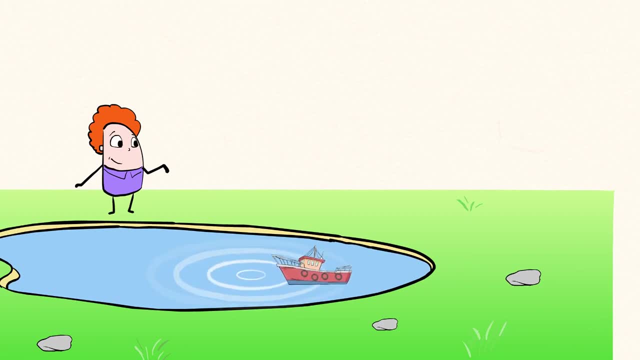 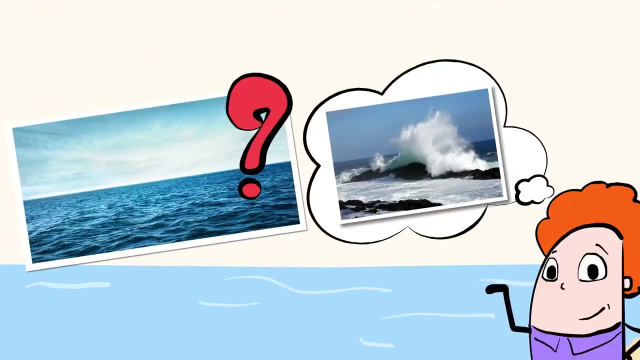 way that sound waves move through the air. The person on the left initiates the wave when they move it, Just like the pebble being thrown in the water started the waves in the pond. Then the wave continues from that point and travels all the way to the other side. Sound waves are longitudinal. 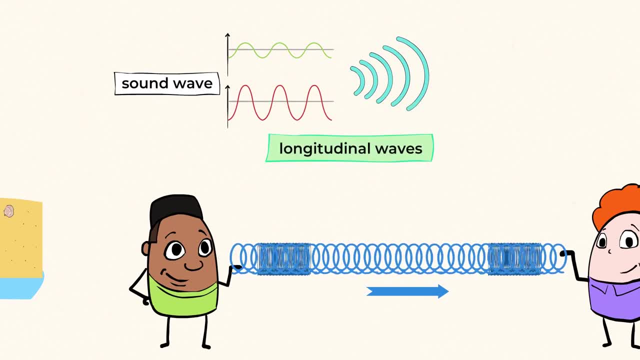 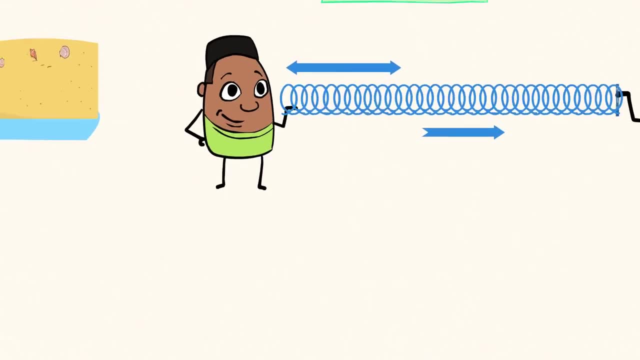 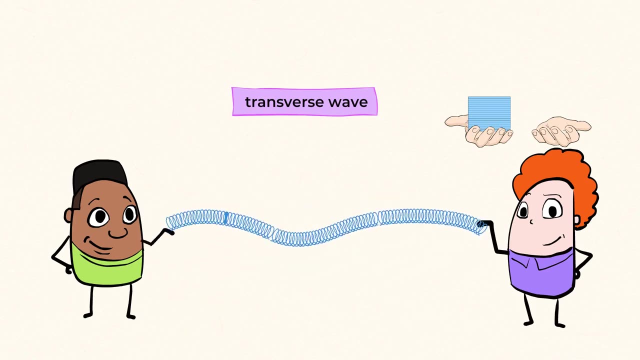 waves, which means they move in the same direction as the disturbance that caused it. In this case, the person moving the end of the toy is causing the wave. But we can also use this toy to show a transverse wave, like a sound wave. A transverse wave moves perpendicular to the disturbance that 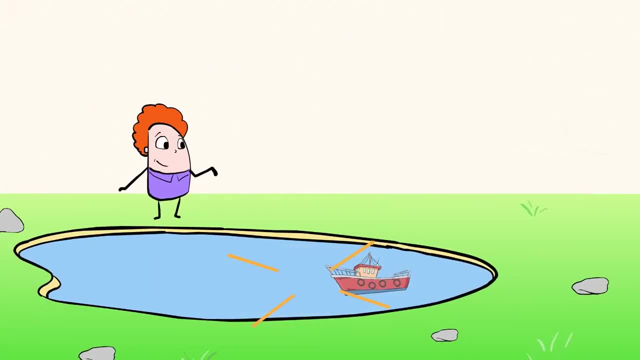 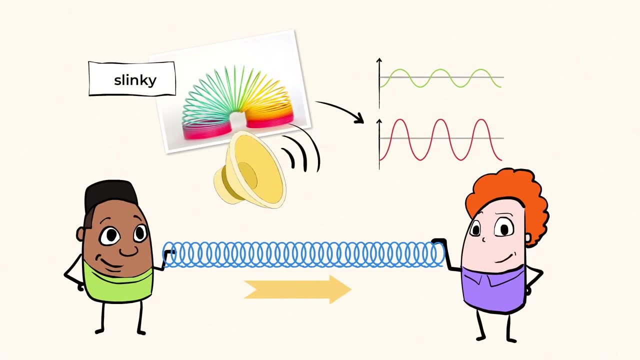 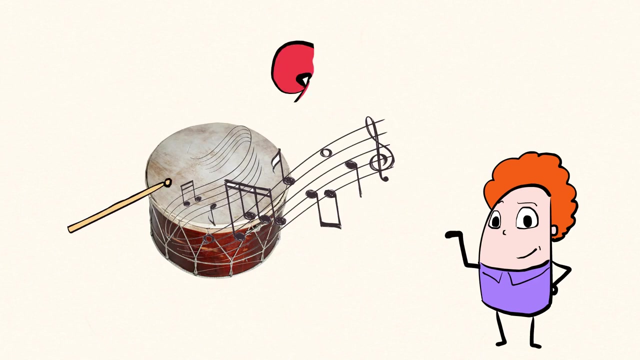 caused it. Remember the pebble we threw into the pond? Those ripples are an example of a transverse wave. All this information is useful for understanding things like sound waves. So turn on the music and let's make some mighty discoveries. This drum is making sound, But how does a drumstick hitting the drum create? 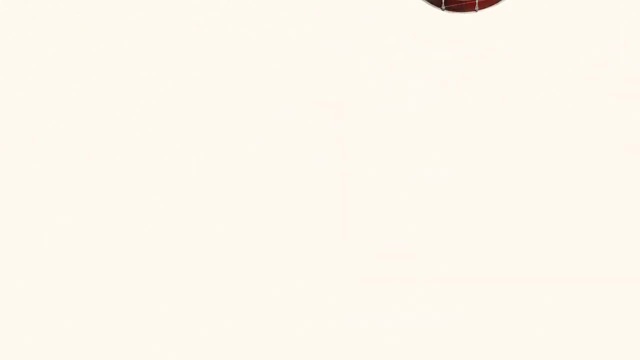 what we hear. It's all about the waves. When the drum is struck, its surface vibrates. That sends waves of vibrations through the air, which then travel into our ears. Sound waves with low amplitude make softer sounds, while sound waves with a higher amplitude make louder sounds. So